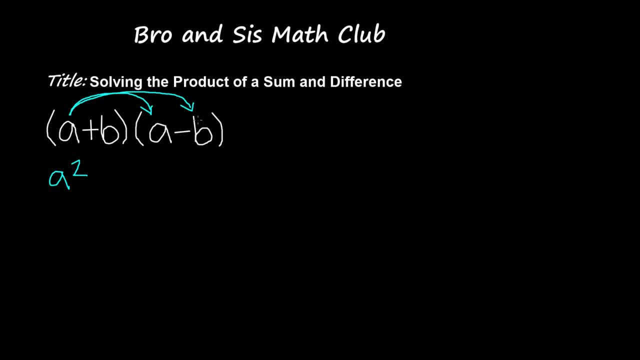 and then we'll distribute a to the negative b, which will give us negative ab, And then we distribute the next term in this binomial alright, which is positive b, to a, which will give us positive ab, and then we're going to multiply b times negative b. 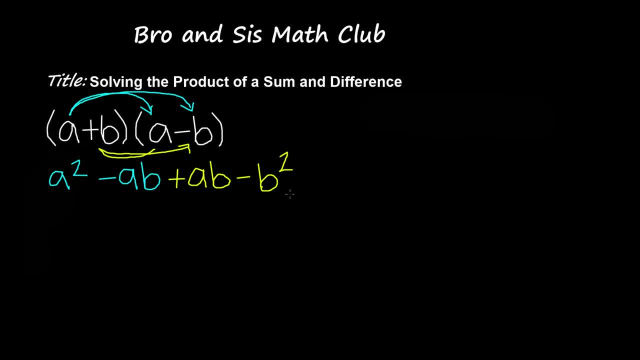 which will give us negative b squared. alright, So when we have a squared, we're going to bring that down, as it is right. and then we see that we have negative ab and positive ab. Now when we have, like, for example, a number that and then we're adding. 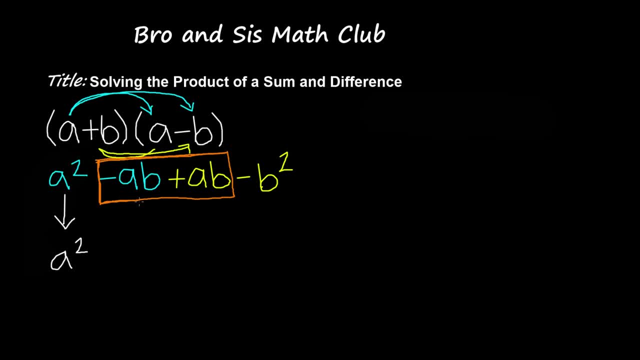 that number to itself, but one is positive and one is negative. what happens is that those two numbers cancel each other out. So same thing happens here. We have ab, but we have one negative ab and we have the other one as a positive ab. 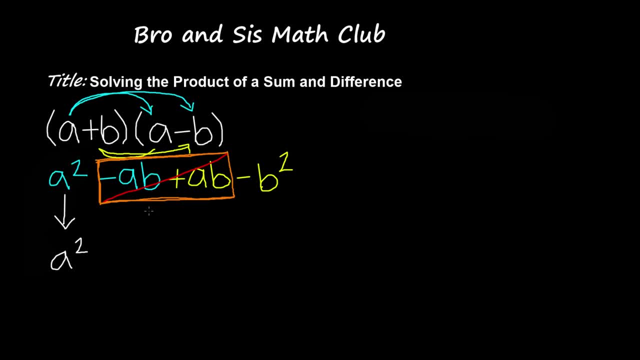 so they're going to cancel each other out, alright, So then we are left with negative b squared. So what we see here is that we don't, we have like no need to do a times b and b times a. 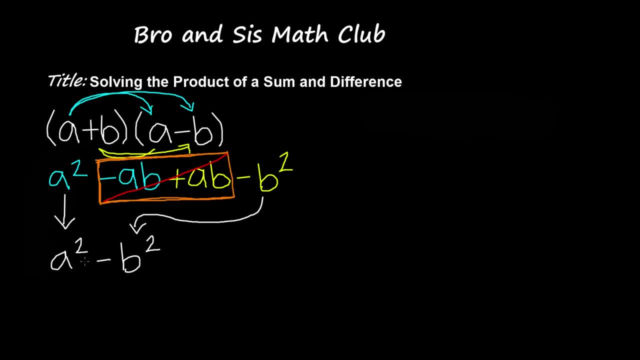 We can simply just follow this shortcut, which is a squared minus b squared. alright, So we're going to do a squared minus b squared. So let's say that we have this problem. We have x plus 9 and x minus 9.. 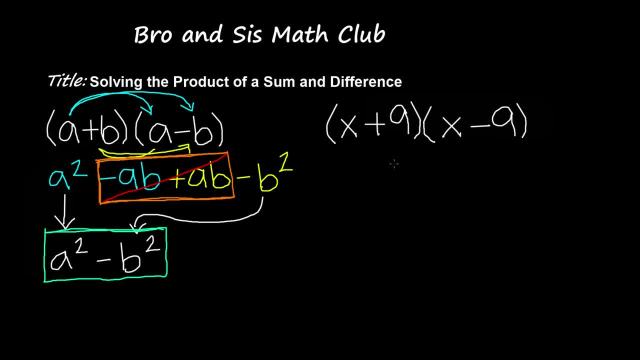 So x is the a and 9 is the b. alright, So we're going to go ahead and follow this method, Which is a squared minus b squared. So I'm going to take the x and square it, and then we have minus. 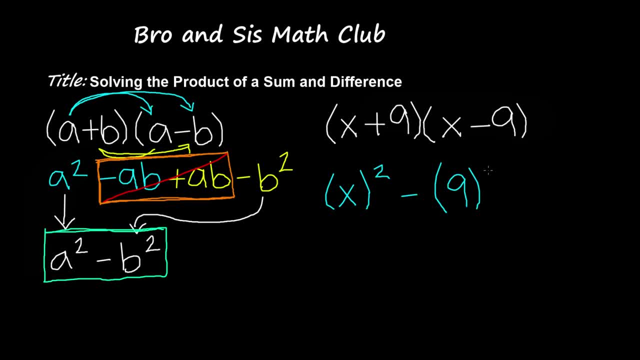 and I'm going to take the 9,- I mean the b, which is 9, and square it as well. So we have, when we have x times x, we get x squared okay, and then subtracted by. and we have, when we have 9 times 9,, we get 81.. 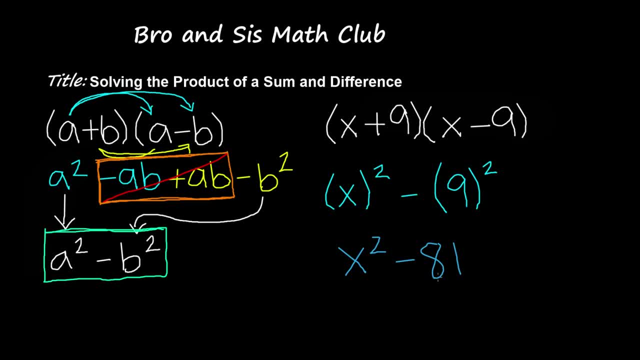 So we get x squared minus 81.. And that would be the answer if you did it the other way. but this is an easier way. It's a. it's a quicker way to solve the product of a sum and difference. alright, 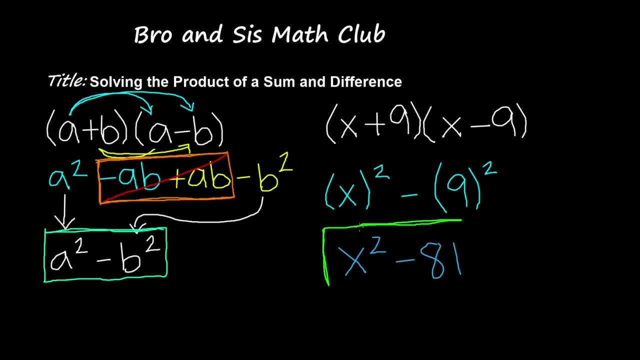 So this is how you solve the product of a sum and difference. Thanks for watching this video and I'll see you guys next time. Bye.